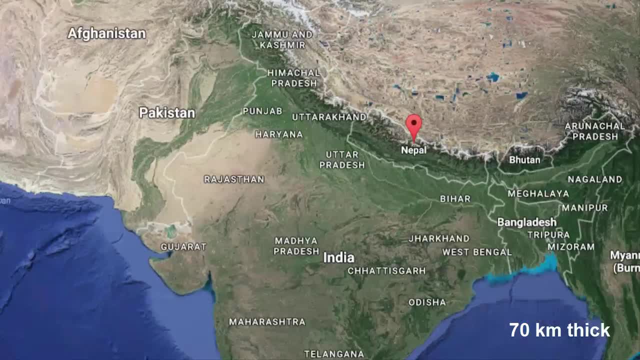 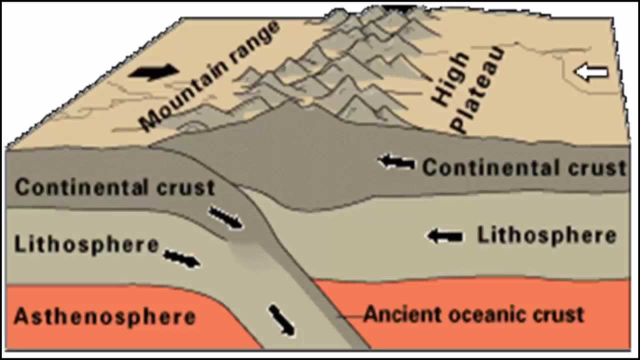 It is as much as 70 kilometer thick in the Himalayan region. Again, we know that Himalaya was formed due to the collision of plates. When two continental plates collide, it folds the rocks at the boundary, lifting it up and leading to formation of mountains and ranges. Therefore, 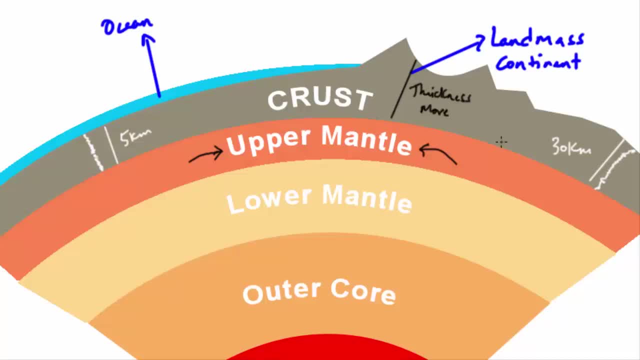 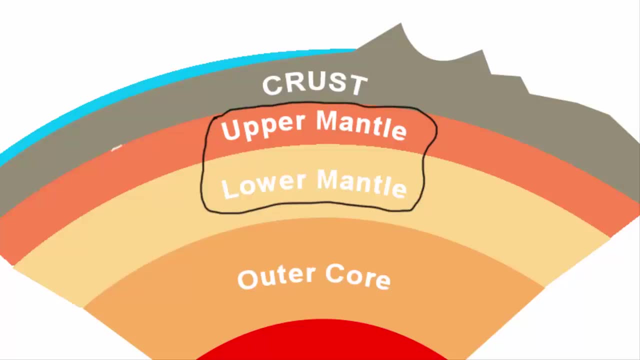 the thickness of the crust in these regions will be naturally higher. The second layer is the mantle. This region over here is called as the mantle, So right from the end of the crust till the outer core is a region that is 2,900 kilometer thick, The upper portion. 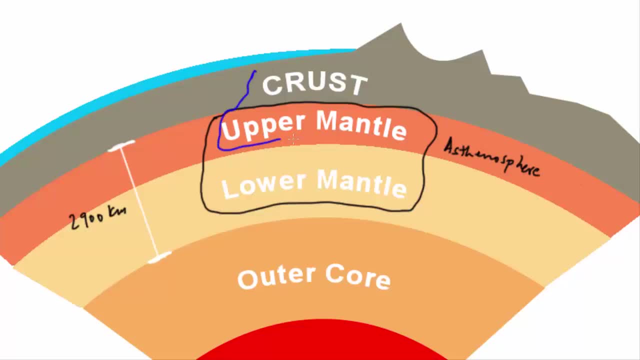 of the mantle is called the upper mantle. This is the upper portion of the upper mantle. This is the upper portion of the upper mantle. This is the upper portion of the upper mantle. This is the called asthenosphere. but this region and the crust together is called lithosphere. 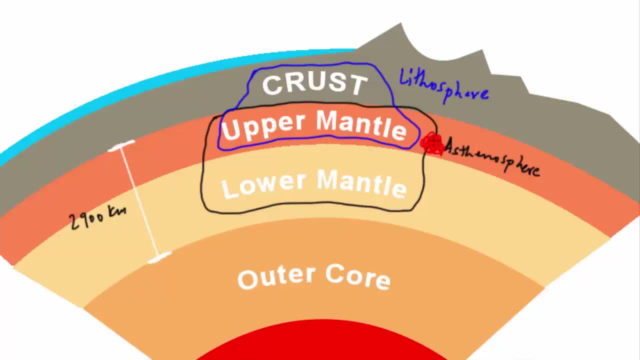 Astheno means weak, and due to its weakness, the magma finds way to the surface during volcanic eruption. Now, the total thickness of the crust and upper mantle, which is also known as the lithosphere, is 200 km. The lower mantle extends beyond the asthenosphere and 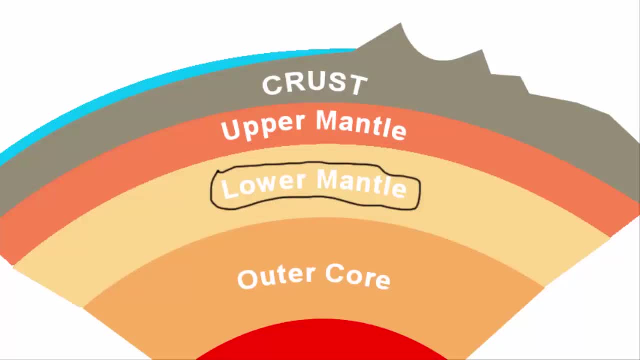 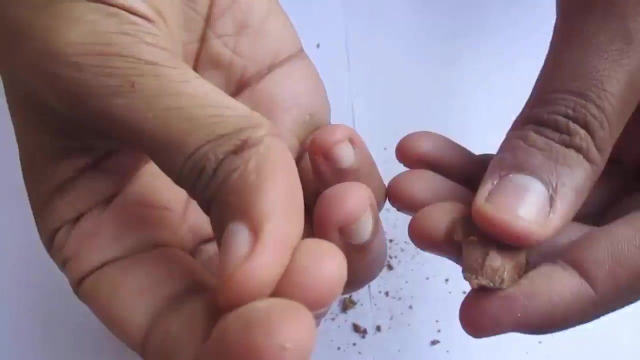 it is in solid state. This layer is also responsible for all of Earth's volcanic and seismic activity, because 2,900 km thickness is pretty spacious area for the formation of such natural catastrophes. Now, laboratory experiments on rocks and minerals say that between 100 and 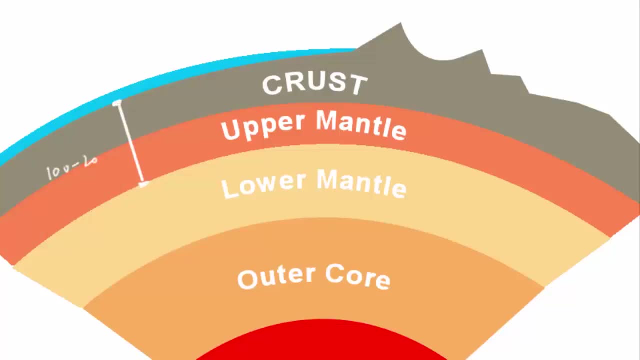 200 km below the Earth's surface, the temperature of the rock is near the melting point. Therefore, molten rock erupted by some volcanoes originates in this region of the mantle. Remember this: the core of the Earth consists of nickel and iron, but here in the mantle it. 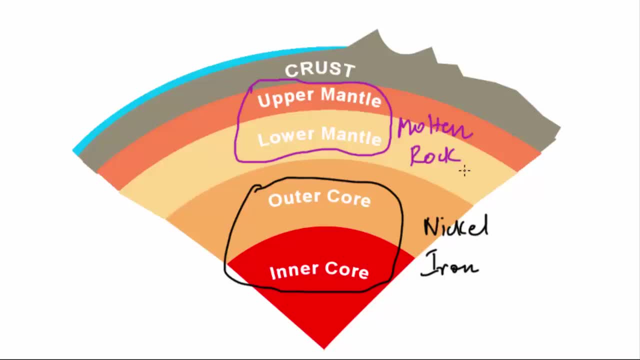 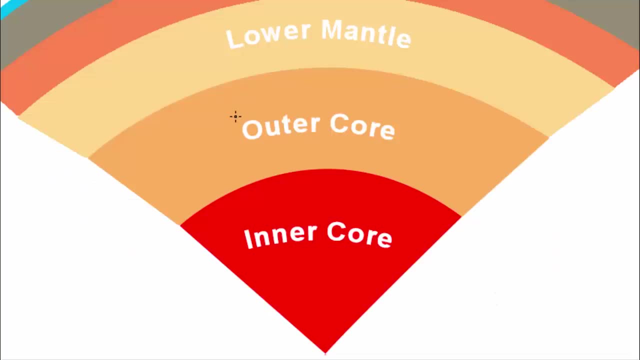 is not. It is the molten rock that is fluid and can move. It is this fluidity that powers the movement of the tectonic plates of the Earth's crust. The third and the final layer is the core. Core comprises of the inner as well as outer. 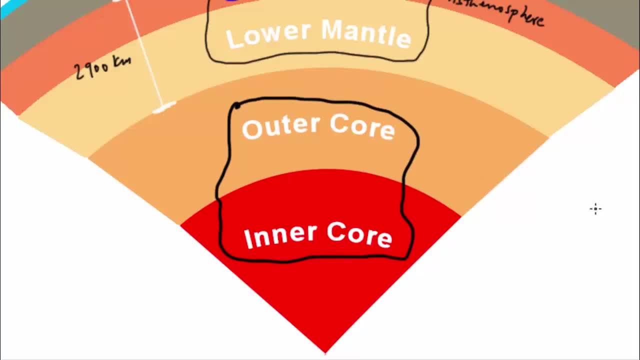 core. Now, moments back, we have read the thickness of the mantle is 2,900 km, So after that, immediately, the boundary of outer core will begin. The outer core is in liquid state, while the inner core is in solid state. I have made a short video on this curious question, If at all you are interested in.